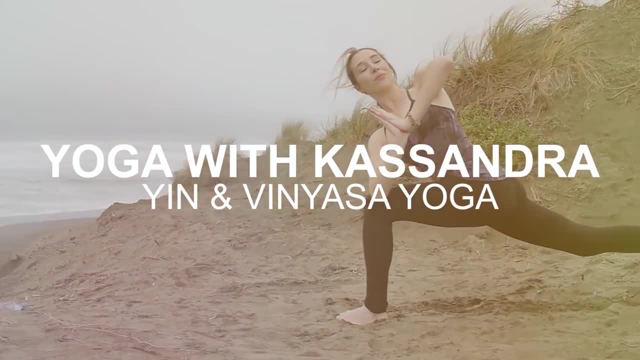 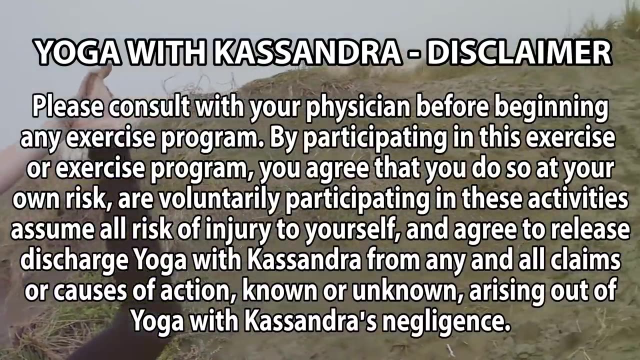 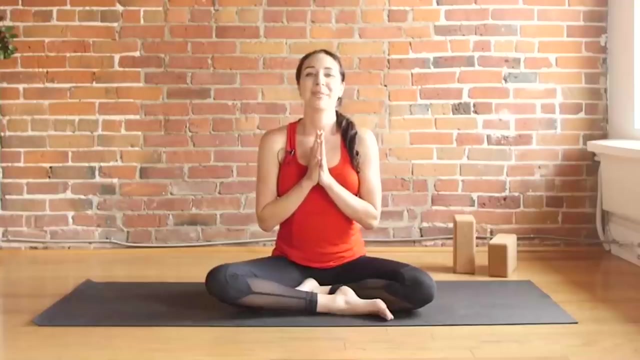 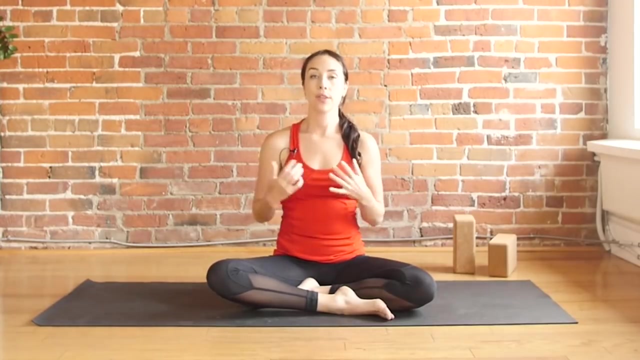 Namaste, Welcome yogis. In today's yin yoga practice, we are going to focus on the spine, So this practice is great for anyone who wants to improve their posture, but it's also a very beneficial practice if you're trying to get into some deeper backbends or some deeper forward. 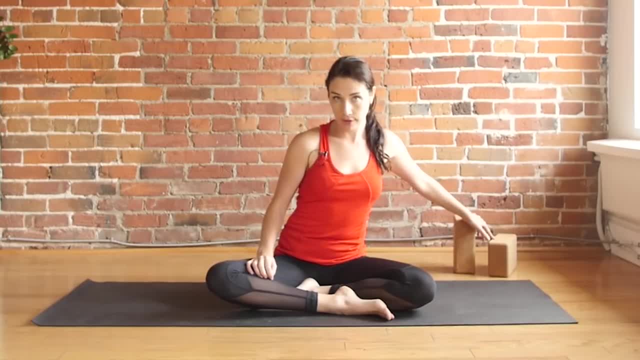 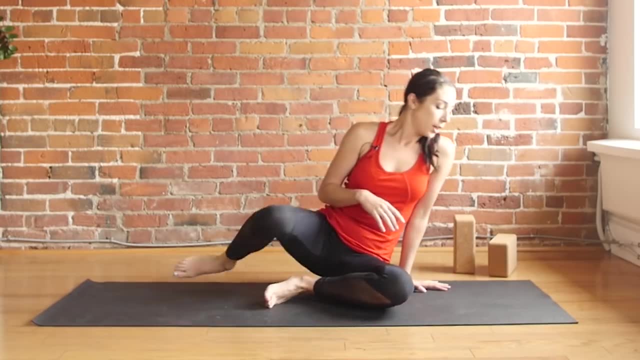 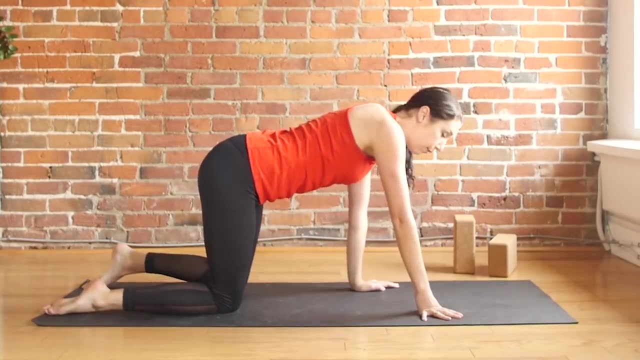 folds. So I'll ask that you have two blocks somewhere close by and our first asana that we will begin in is melting heart or puppy pose. So, starting on your hands and knees, you're welcome. Feel free here to prop something underneath your knees if it's hard, and 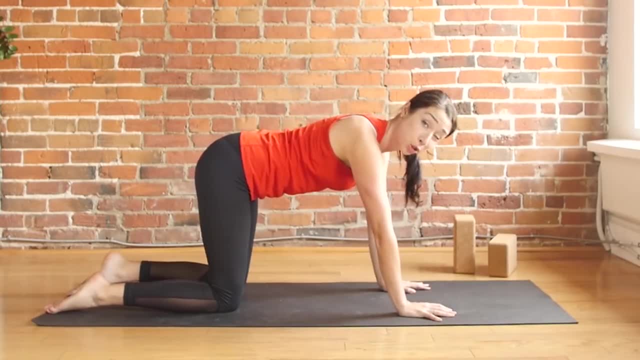 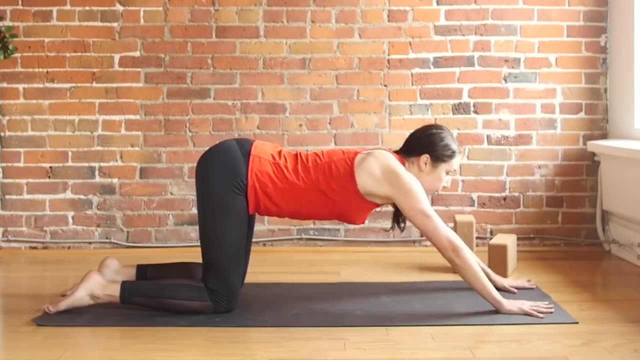 uncomfortable to stay this way. You can either fold up your mat or just put a blanket there. Hips need to be directly over the top of your knees and you're simply going to walk your palms forward until the forehead and the chest can melt down to the mat. Now having the arms, 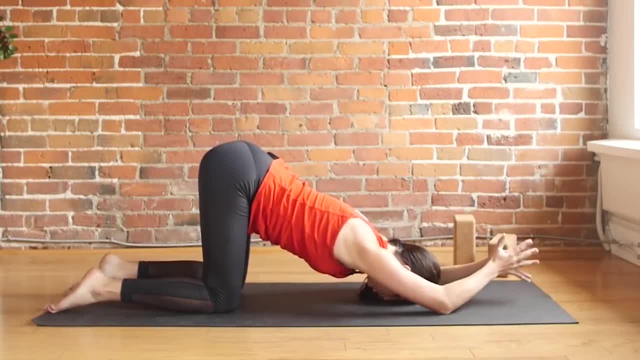 extended is your first option. Another option you might enjoy would be to press the palms together and to bring the thumbs towards the back of the neck and the back of the head. This will go a little bit deeper into the triceps and into the chest, So it just depends on. 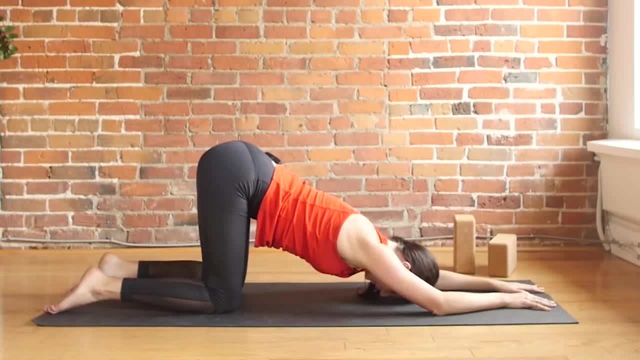 what feels best for your body today And while the belly does drop to the floor here in a pose like this, try to draw the low belly into the low back so you're not hyperextending too much through the low back or not pinching and compressing this area. We're really instead, 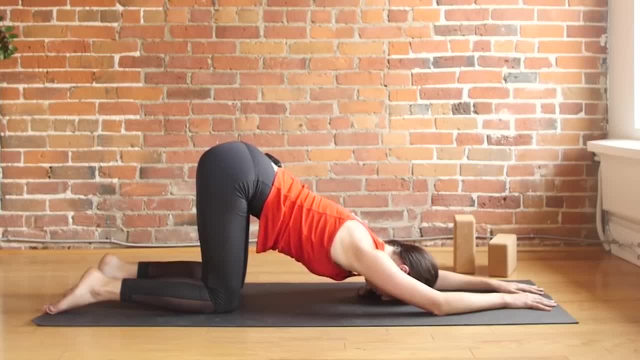 trying to focus on the upper back and upper body. Draw your shoulder blades down your back, relax your neck and just breathe, And then you're going to come back into the space you're creating, Feeling the rib cage expand front to back and side to side. 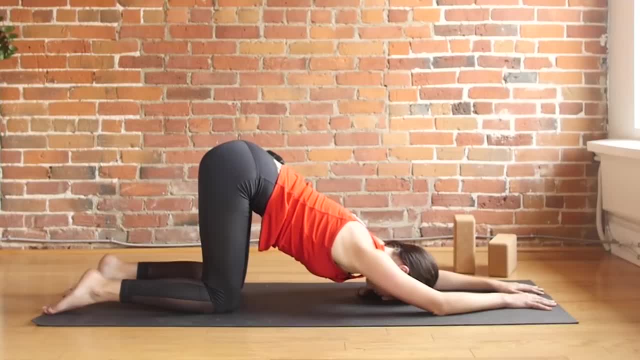 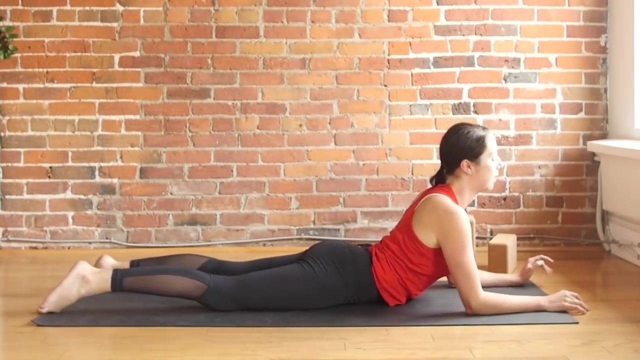 Thank you, Thank you, Thank you. And let's slide forward onto our stomachs for Sphinx Pose. So pelvis is planted down to the floor And you can widen your elbows and your palms lifting through the chest and through the heart. 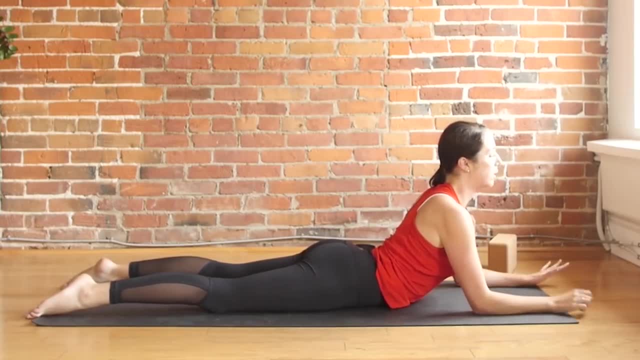 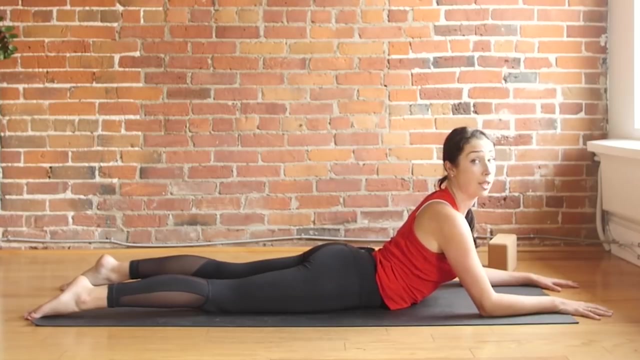 So think of drawing and pushing your shoulders back, squeezing your shoulder blades behind you as you pull your heart forward And breathe into the front of the body, And if this feels like too deep of a backbend, you can always walk your arms further out in front of you to lessen the intensity of the pose. 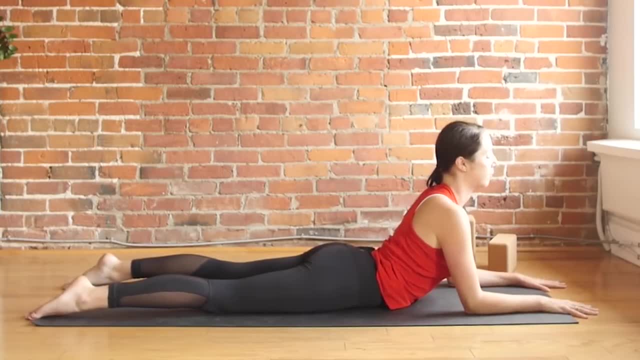 Otherwise, stay tall and lifted. Sphinx Pose. Sphinx Pose consisted of 4 circles in a Masters pose position. Treat in the same way as obesession and exercise. Make that pause longer, for 3 or 4 seconds at a time. In this time, better understab yourself and avoid movements that exercise the chest muscles. 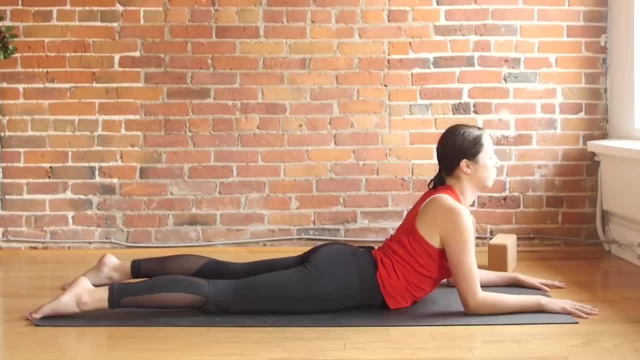 To apply it back in to the front of the body without touching the skin. Join-up of hugs and turns. Place your universen and close your eyes, cleaning up the past. Draw and lift your shoulders back and forth. Breathe it in. 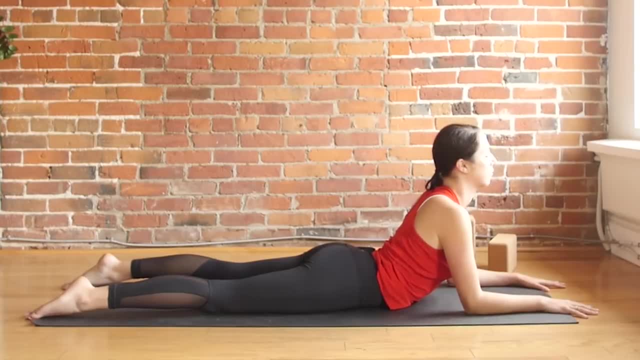 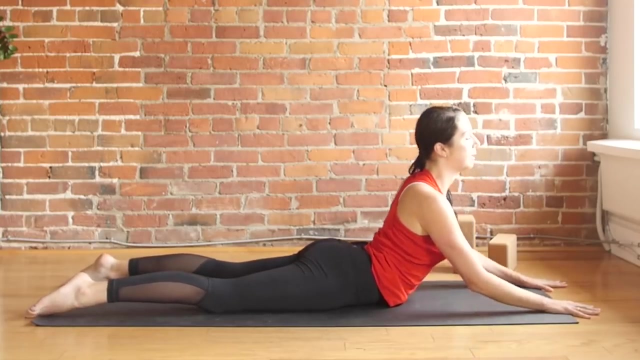 Relax and breathe out. Close your eyes and relax. Just close your eyes, Relax and you're welcome to stay here for the second half of our time in this pose. or you can progress a little bit deeper by lifting up into seal, so pressing the arms straight. 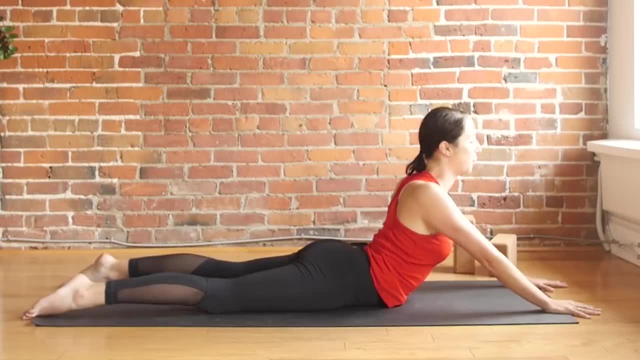 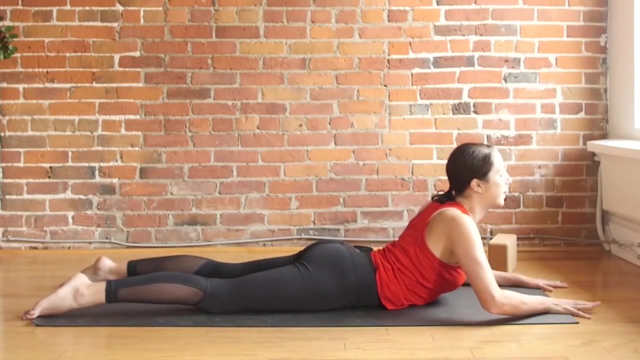 if this hurts your lower back, come back down onto your forearms. if this hurts your lower back, come back down onto your forearms, bend the elbows. if you were in seal, and let's bend the elbows if you were in seal, and let's bend the elbows if you were in seal, and let's press. 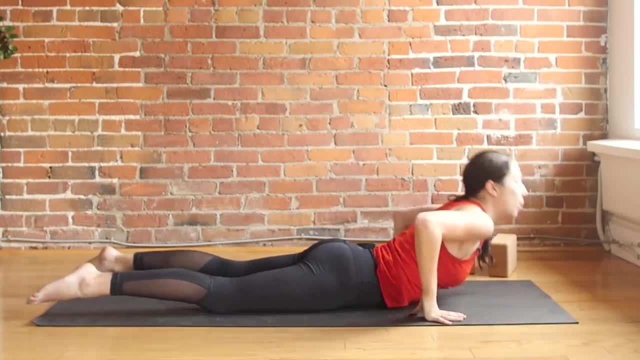 bend the elbows if you were in seal and let's press back into an easy child's pose, back into an easy child's pose, back into an easy child's pose, one of the most nurturing asanas we can. one of the most nurturing asanas we can. 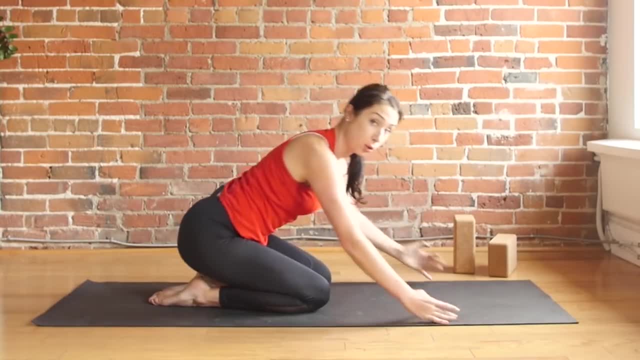 one of the most nurturing asanas we can do for our spine, and so keeping the do for our spine and so keeping the do for our spine, and so keeping the knees pretty close in towards each other, knees pretty close in towards each other, knees pretty close in towards each other as you bring your hips to your heels. 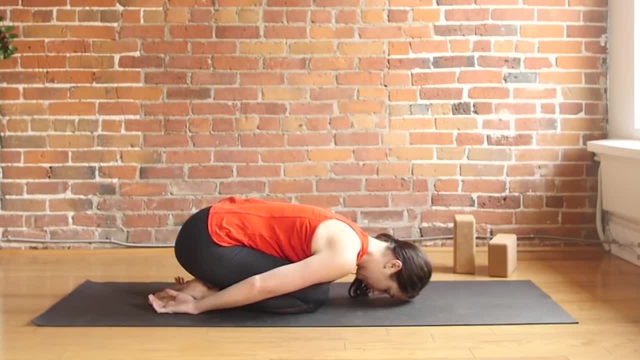 as you bring your hips to your heels, as you bring your hips to your heels, arms extend back forehead down to the arms. extend back forehead, down to the arms. extend back forehead down to the mat. so letting your spine naturally mat. so letting your spine naturally mat. so letting your spine naturally curve. here, arms are heavy by your sides. 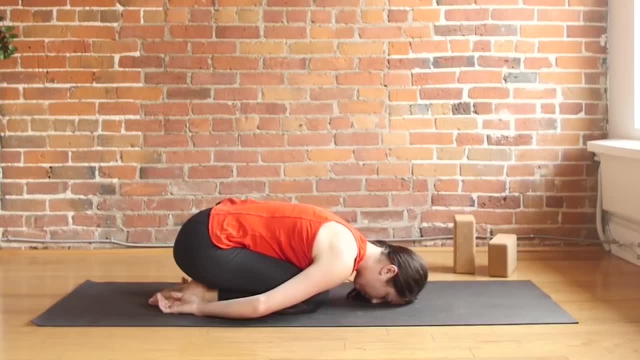 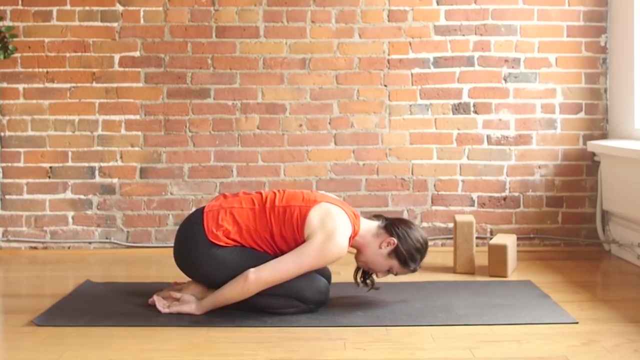 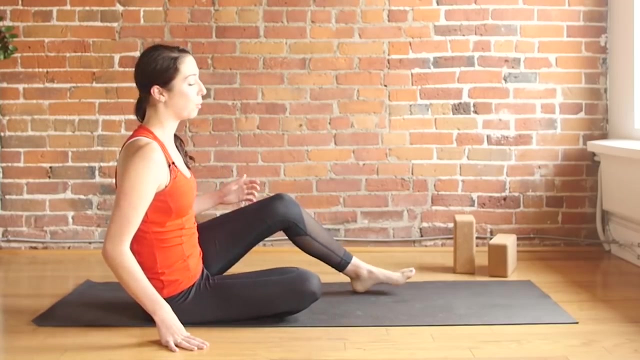 curve here. arms are heavy by your sides. relax fully in this pose, breathing into the back body. relax fully in this pose. relax fully in this pose. let's roll up. now you can bring your legs out in front of you. we'll make our way into caterpillar, which is a forward fold, so feet are about hip-width. 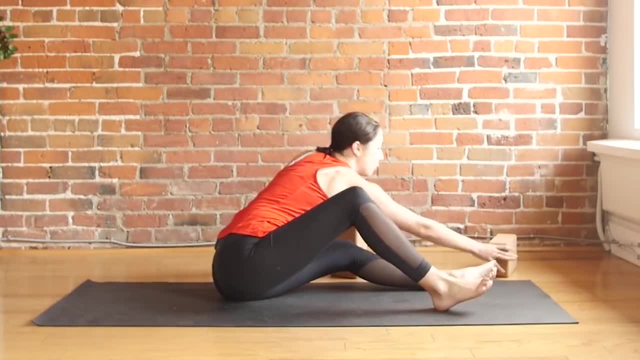 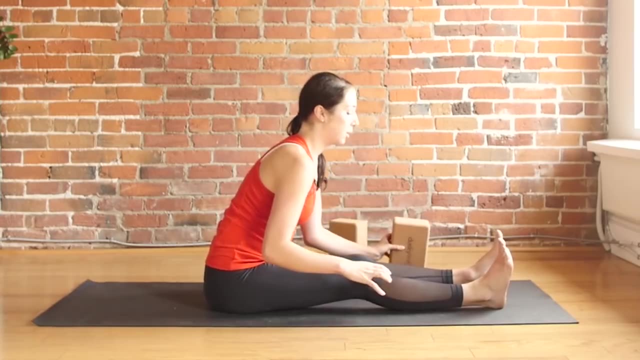 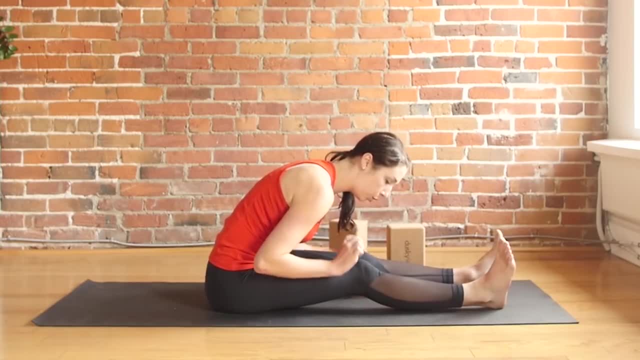 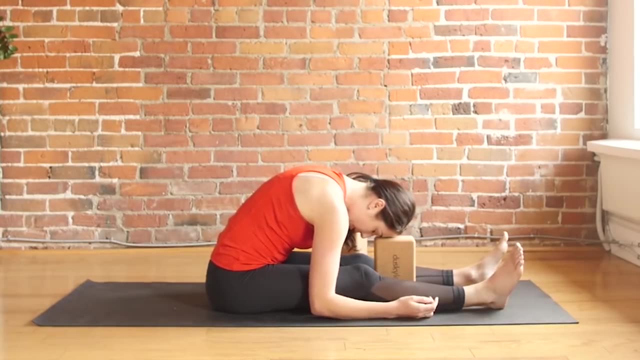 a little bit of a bend is perfectly fine here in your knees. you don't want to hyper, extend or lock into the joints and you could choose to just let your head dangle and gravity will slowly lower you into the pose. or if you're somewhere close, you can always use a block or two stacking them underneath. so 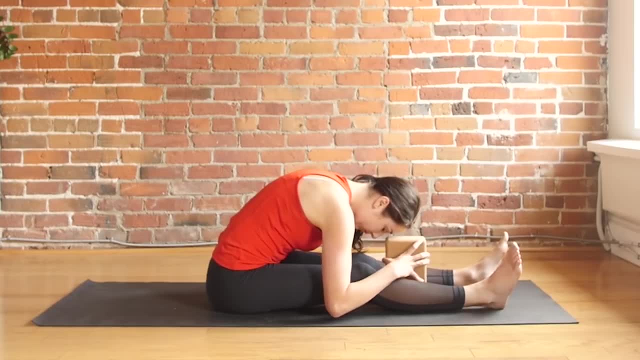 that you have something to rest on, and I like to turn the palms to face up so that I'm not tempted to push or pull. we really need this, this fold, to be passive. so gravity is doing the work for you and this is an intense asana for the spine. can you breathe into it as if you? 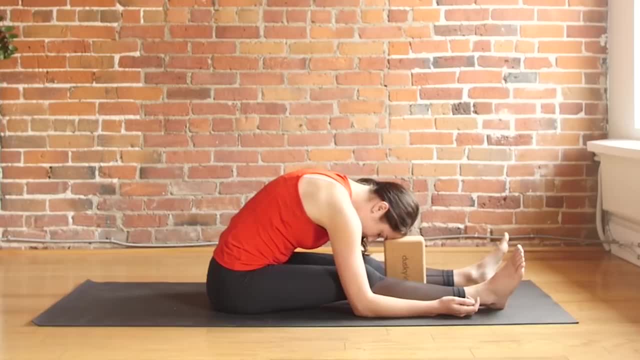 could breathe into every single vertebrae, engaging the entire posterior chain or stretching the entire posterior chain. so, from the crown of your head all the way down through the neck, the spine, into the back of the legs and the soles of the feet, you, you, you. 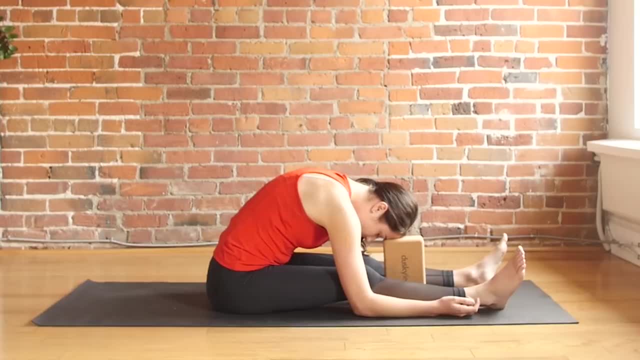 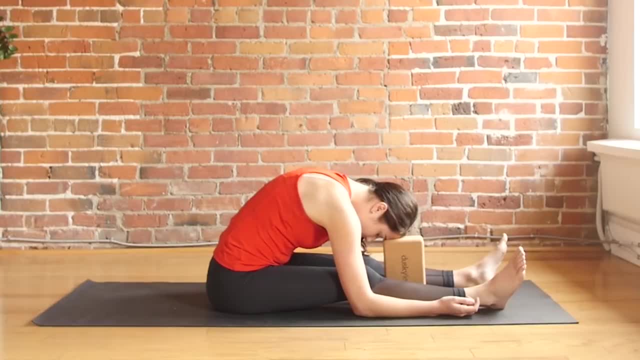 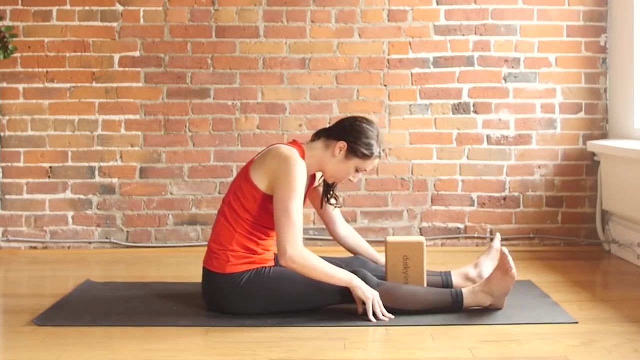 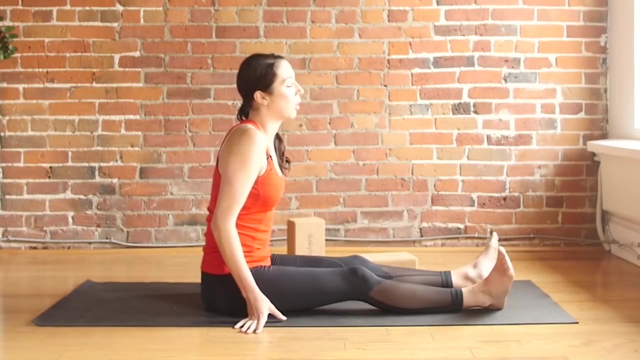 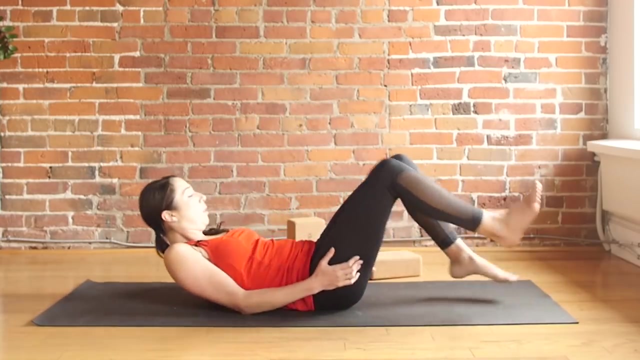 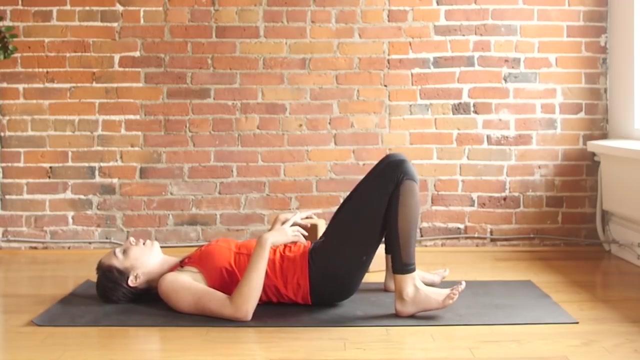 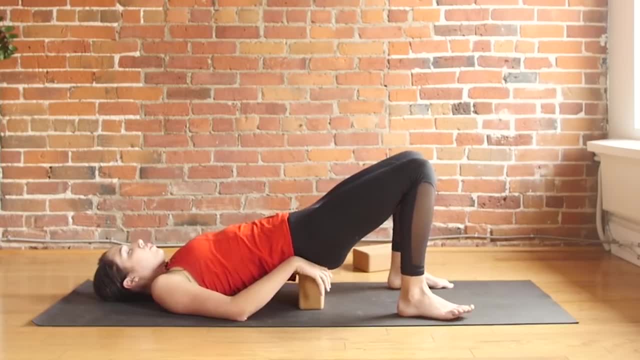 And you can put your block underneath the hips, underneath the tailbone, either on its second or first height, really whichever height feels the most comfortable and the best for you. First option is to keep your knees bent and your feet flat on the floor. 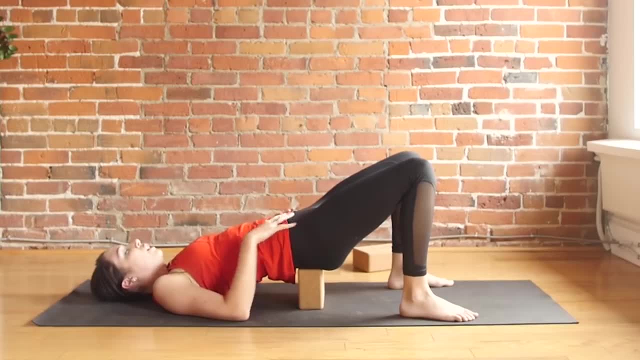 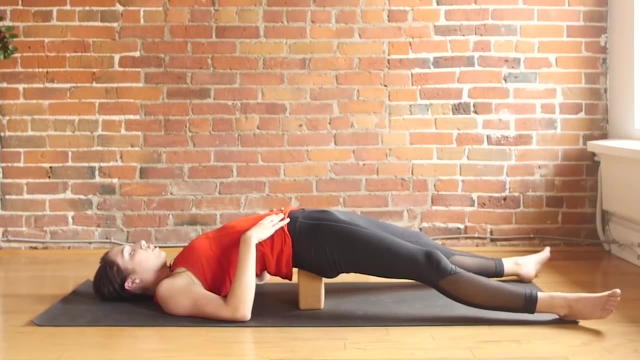 This is a great way to recalibrate the spine. If you'd like to get into the hip flexors, you can extend both legs out in front of you. Just make sure it doesn't compress your lower back or cause any kind of pain in there. 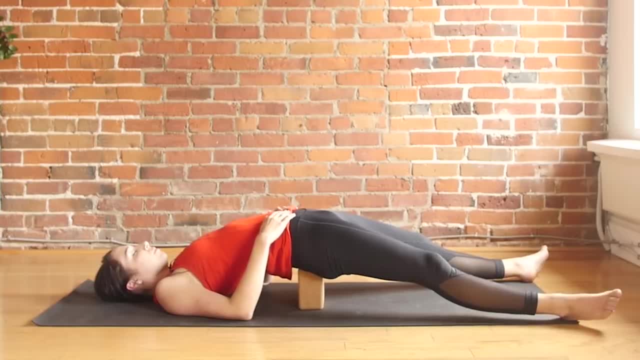 And this way you can keep your back straight as you put your legs out And you can stretch your body out into the mat. And you can do this as you aren't with your legs out. We do this with the back of the hands. 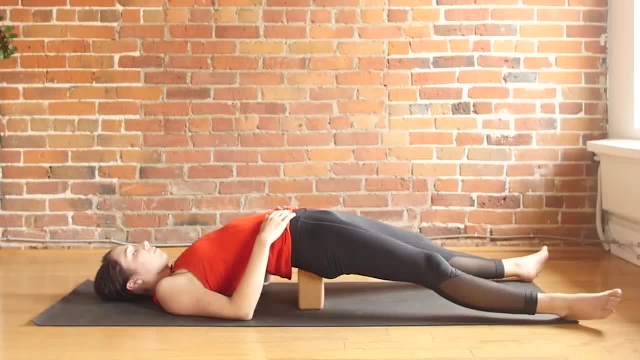 Walk your feet right down to the mat And you can just stretch your back to the back, just like this. Now we are all on the same leg And I want you to keep your feet straight. You don't want to tilt your head back. 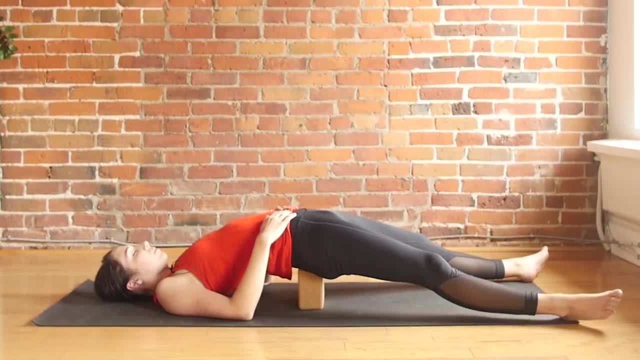 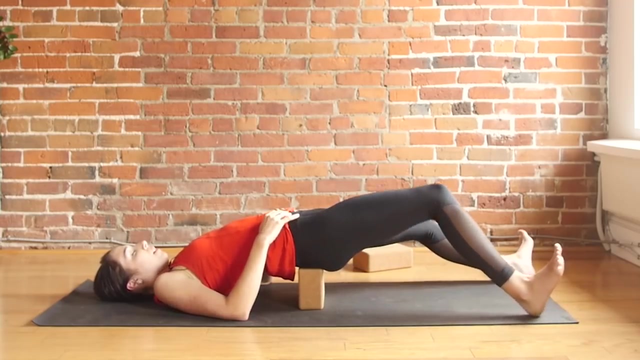 Make sure your lower back and knees are in the same position. Thank you, Thank you, Thank you. If you had your legs extended out in front of you, you can bend the knees one at a time, And we're going to push into the feet to lift the pelvis. 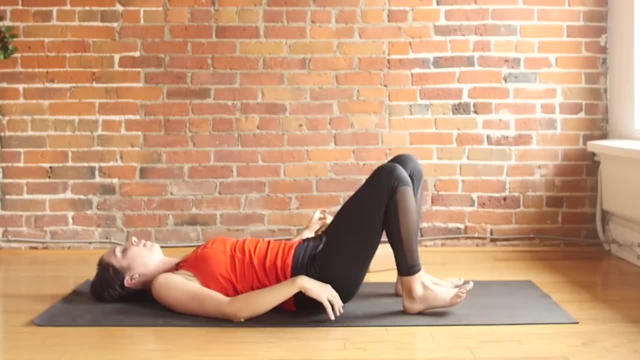 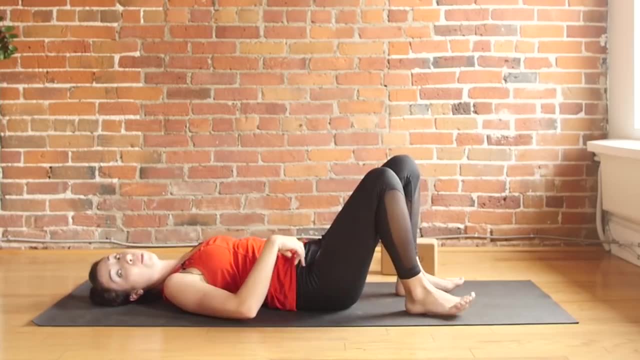 and move the blocks out to the side. We won't need them anymore. And before going into Shavasana we'll take a lying spinal twist, a great counter pose after all of those More intense yin poses, So arms can reach out to the sides. 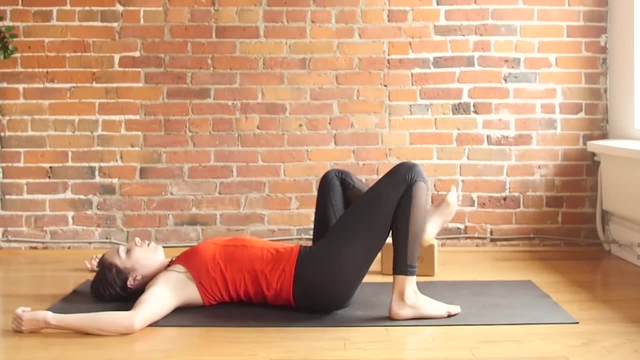 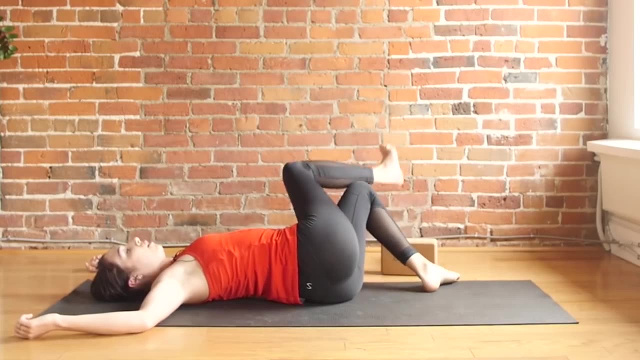 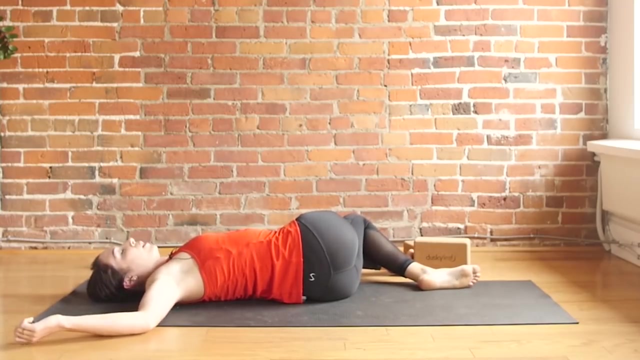 and you can move your hips a couple inches to the right before letting both knees drop down over to the left, Either keeping one thigh stacked over the other, or you can wrap your right leg over the left one before letting the knees drop. Try to keep your right shoulder blade in contact with the floor. 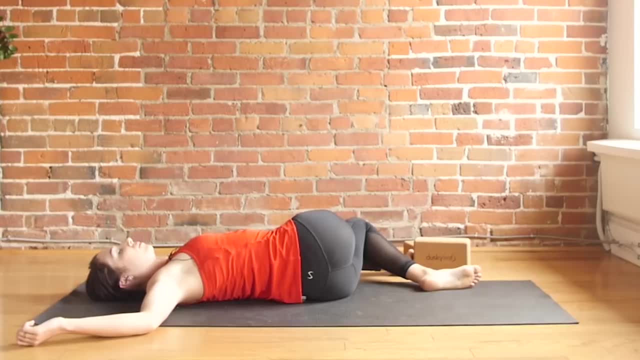 Thin legs And when you sit down straight you can bend the feet to the side And then if you want to try that you can use your right foot to keep your right foot in contact with the floor. So hold it in. Your right leg will have to be in contact with the floor. 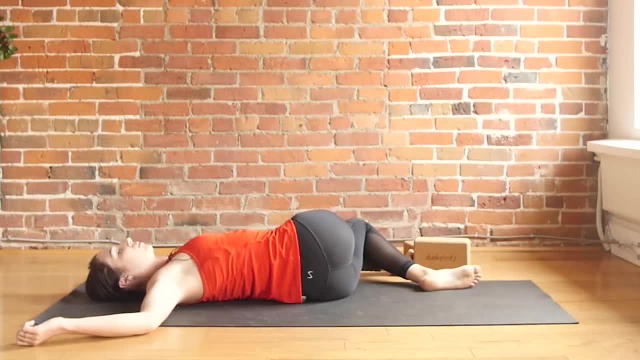 Don't try to lift your body. No, you've got to have the hips in contact. When you lift the feet, you can see your leg And then, if you lift them, you can lift the hips and your hips. You're doing great. 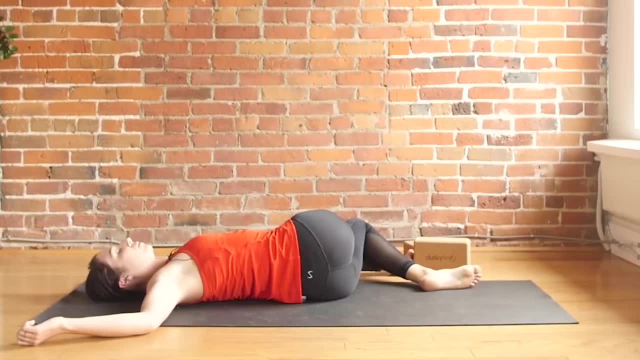 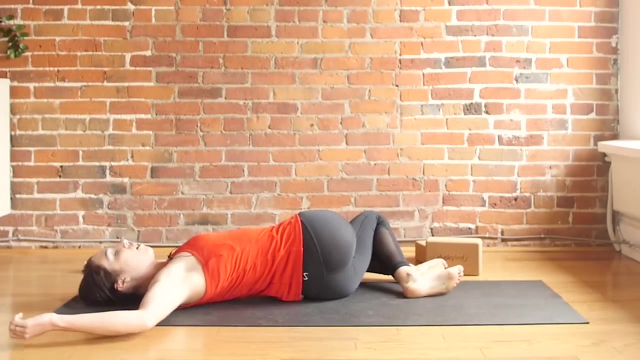 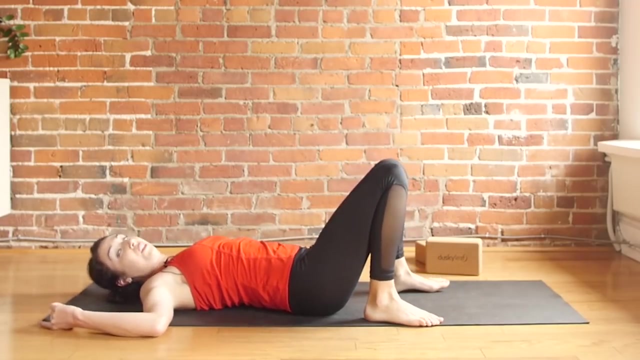 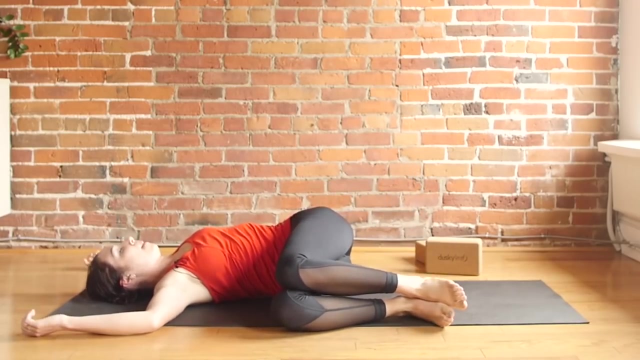 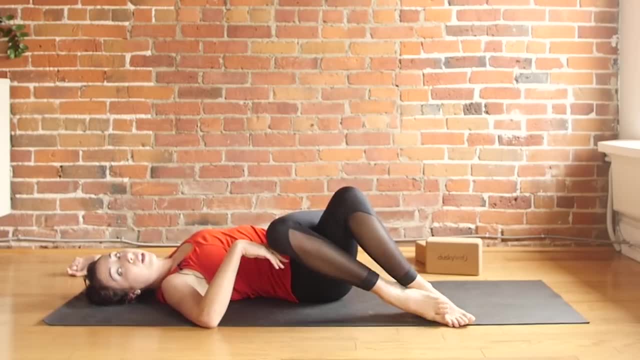 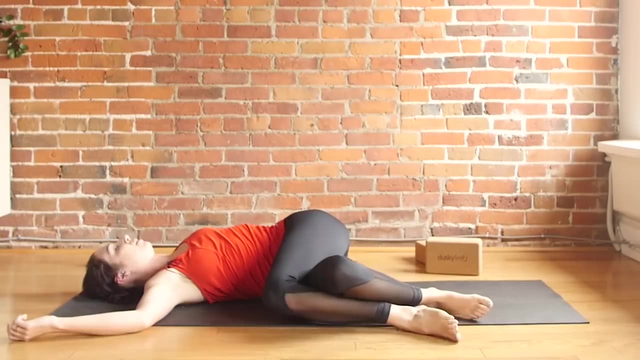 either keeping one thigh over the other or wrapping your left leg over your right one. Try to ground and press your left shoulder blade into the mat. We're creating as much space between the left shoulder and the top of the left hip as we possibly can. 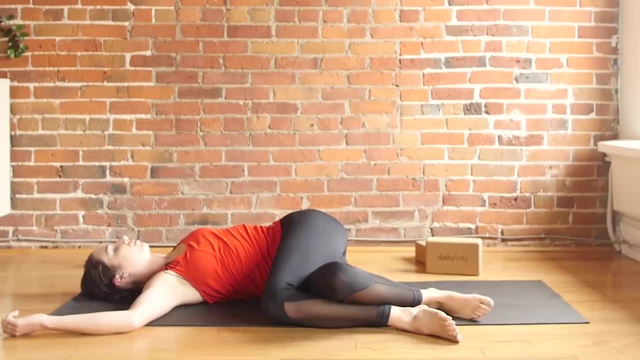 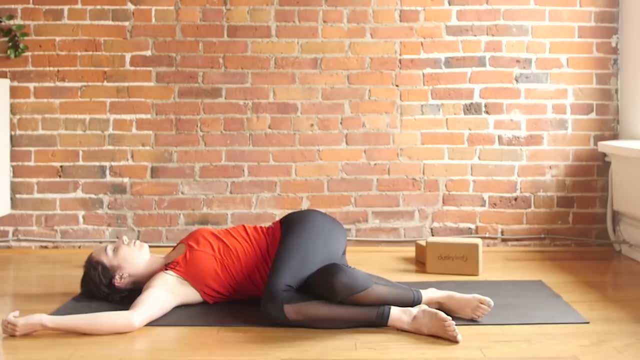 We're creating as much space between the left shoulder and the top of the left hip as we possibly can. We're creating as much space between the left shoulder and the top of the left hip as we possibly can Uncross and unwrap the legs. 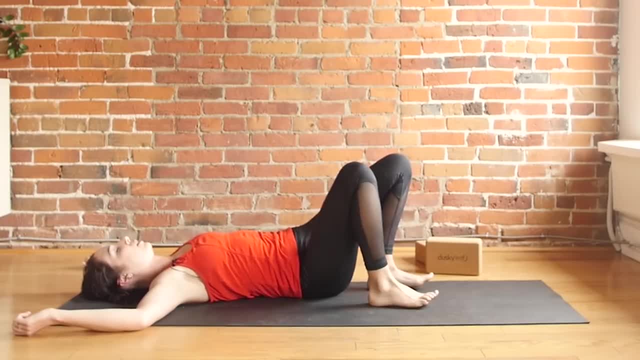 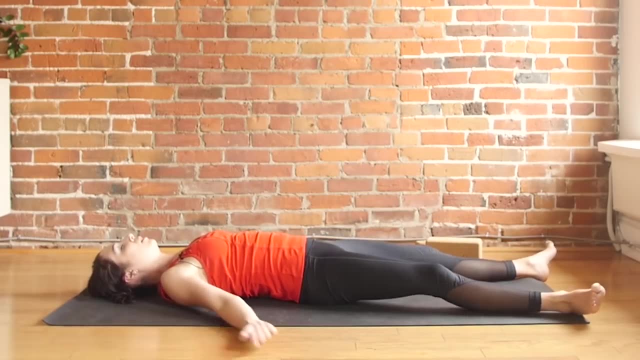 And we're finally ready for Shavasana, our final resting pose. Take up some space, Get comfortable here. Palms face up to the sky, Let your body relax fully with your spine leveled. Just notice the effects of your practice. 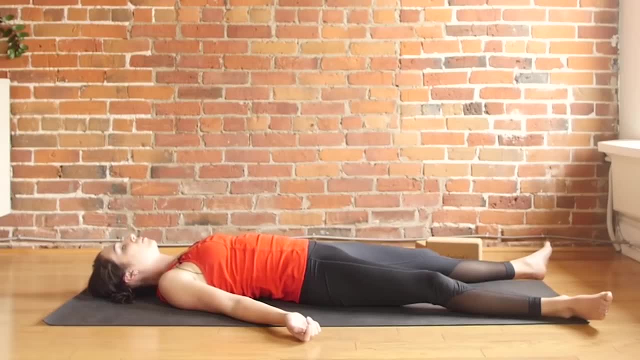 on your spine. let yourself soften here as a way to process and integrate all the work that you've done, giving yourself these last few minutes of silence and stillness. you, you, you, deep in your breath, make movements in the extremities so you can wake back up. 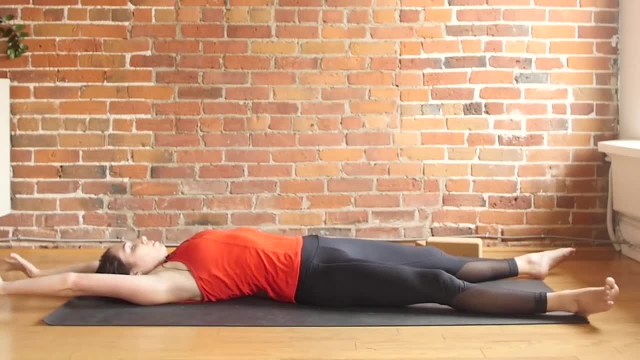 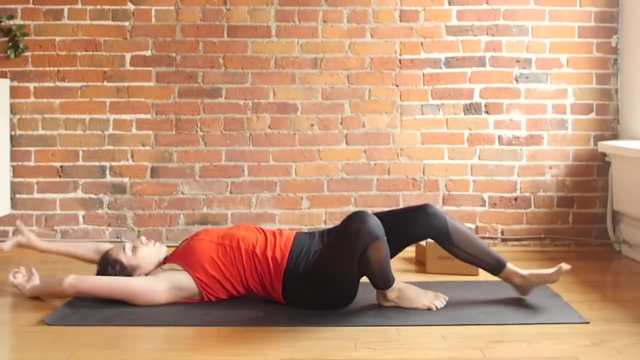 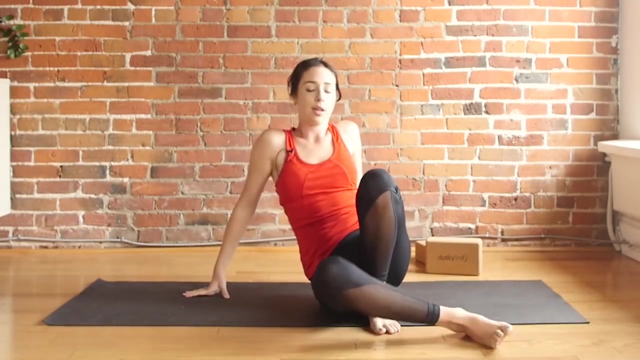 take a great big stretch, lengthening your spine, reaching fingertips all the way down to the toes, and roll to one side, use your arms to help yourself, come up and take a seat. you can keep your eyes closed as you do this, just sitting here, sitting here any way that is comfortable.